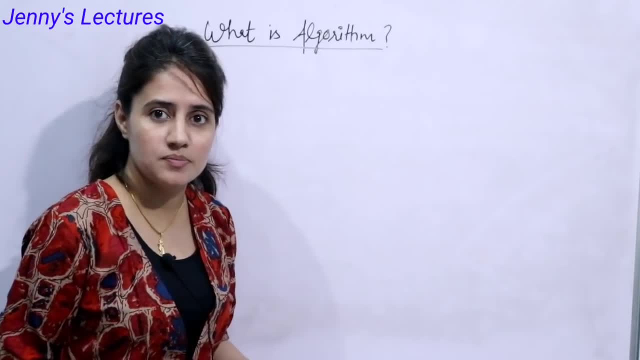 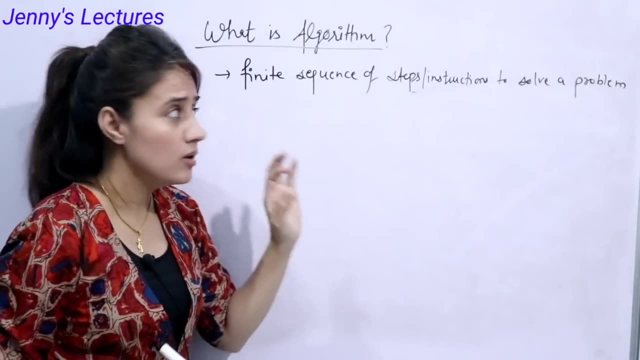 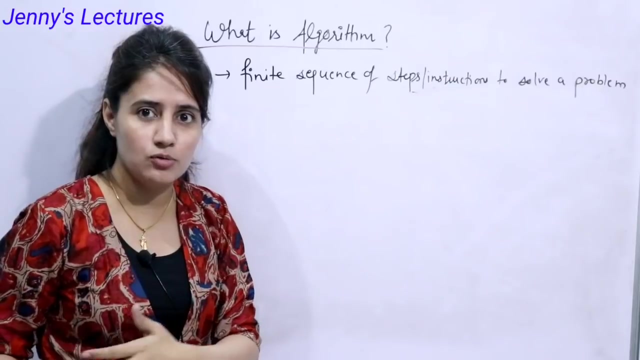 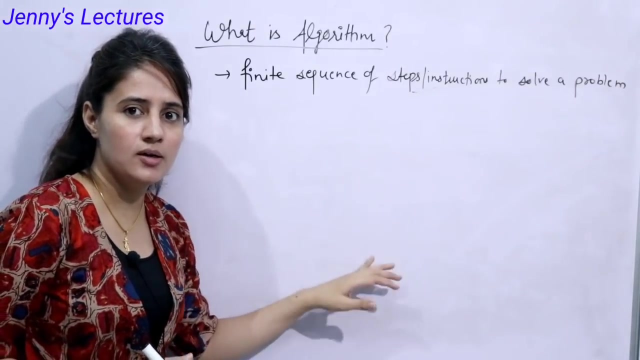 Or you can say: used to solve a computational problem. It is better to say sequence of steps or instructions. Either you can write steps or instruction. Why Rather than set of steps? because in a set we can have same type of multiple values. The values can be repeated. But that should not be a case in algorithm, Like we cannot repeat same step again and again, like read A, read A, read A. One step would be one time, like read A Fine. So 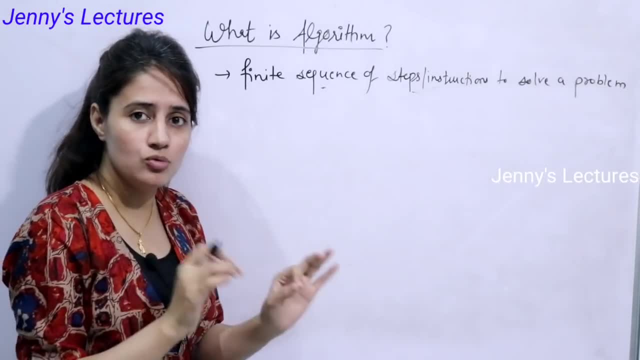 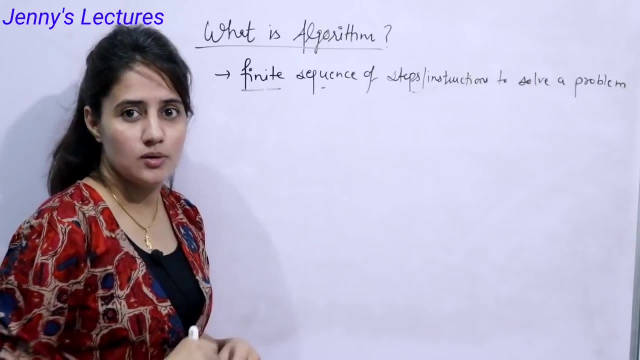 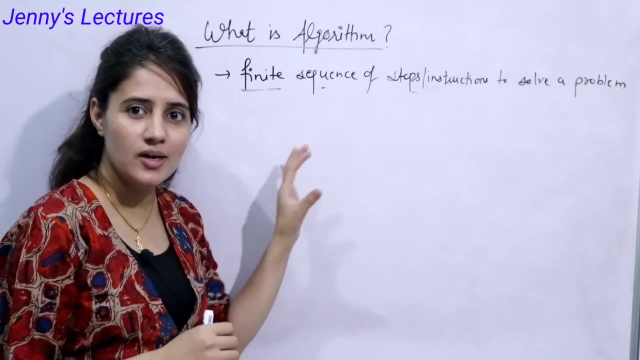 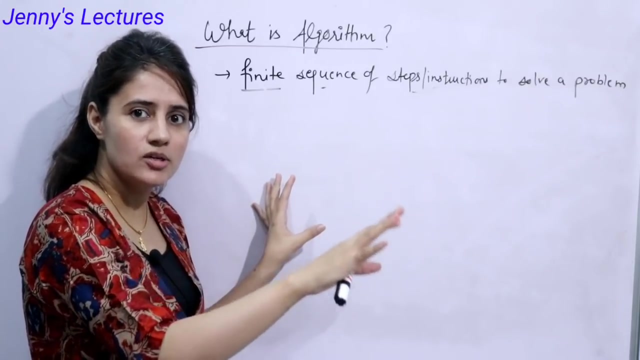 it is better to say sequence of instructions to solve a problem or to solve a computational problem, Right Finite sequence of steps. Now why we need algorithms. Let us take a real life example, Like if you want to construct a building. in that case, first of all, what you will do, Obviously, you design a map and then start construction. If you want some update, then you update that map only and then actually construction should be started, Right, It is not like that: without map, without any planning, without any 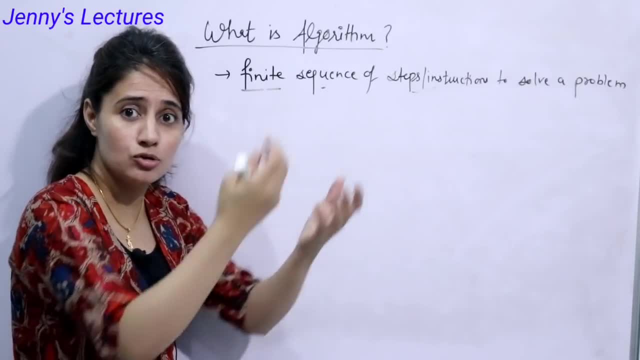 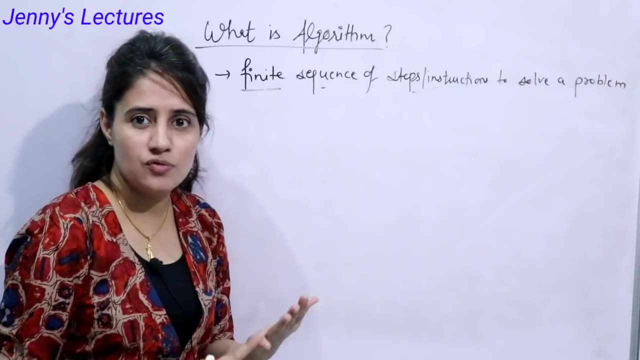 designing, start directly construction. If you don't like anything, then destroy that already constructed building and again start construction. If you do so, then it is wastage of money, wastage of time, right? So that map is what It's. you can say relate. you can say that map is. 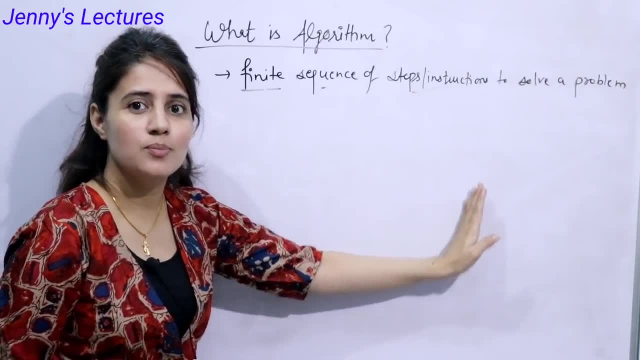 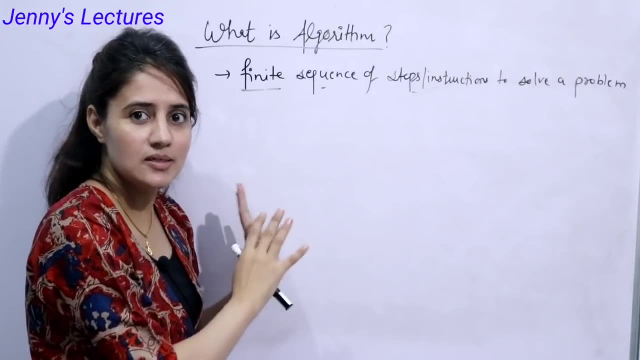 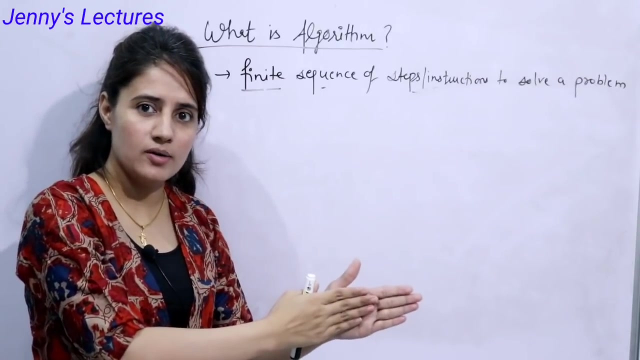 algorithm and the construction. actual construction is what Program? That thing we'll also discuss. So for better construction, map is necessary. So in computer science language you can say: to design a better program, algorithms are required. First of all algorithms are written. 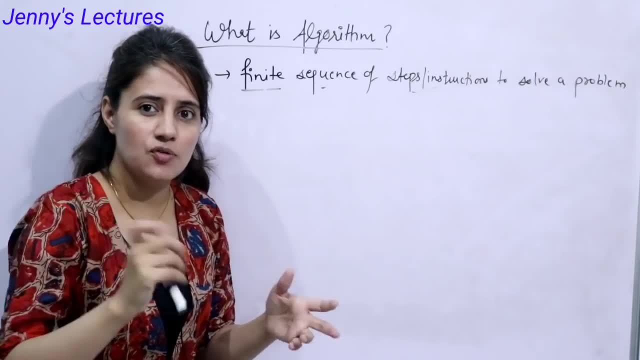 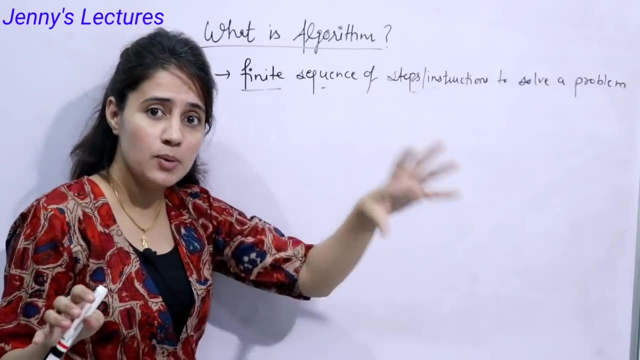 then programs are written, Like: if you have knowledge of SDLC software development life cycle, then first design phase is there right, And then development phase. or you can say the implementation phase, In implementation phase you code. or you can say: the programmers write. 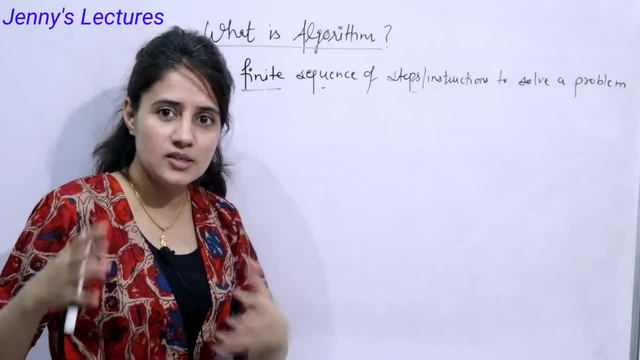 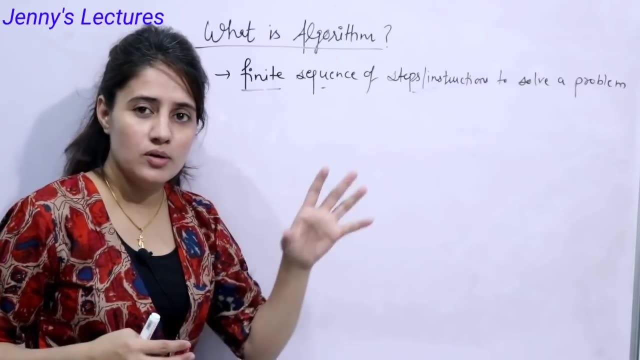 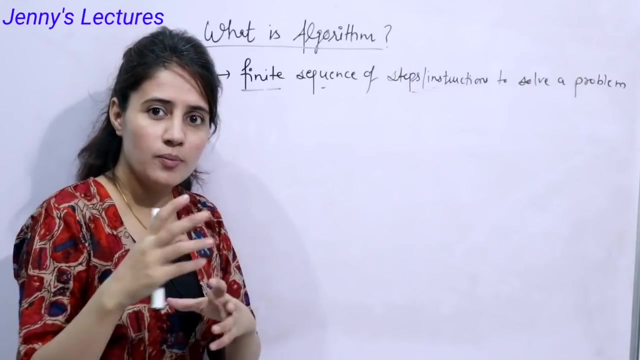 programs And first of all the design phase. In design phase, actually, there we write, they write algorithms. Like suppose, if anyone want to develop a software- it's not like a- directly start writing programs And if there is any mistake or you want to update something, then again write a new program. Fine, No, First of 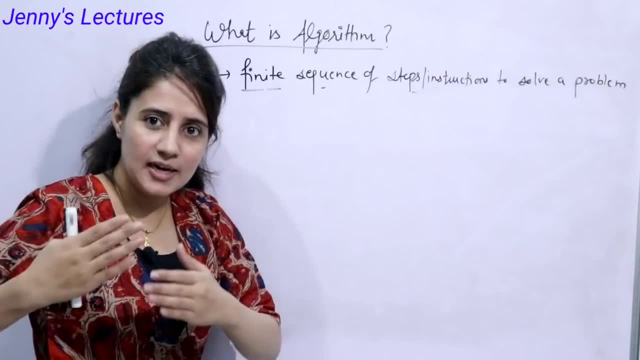 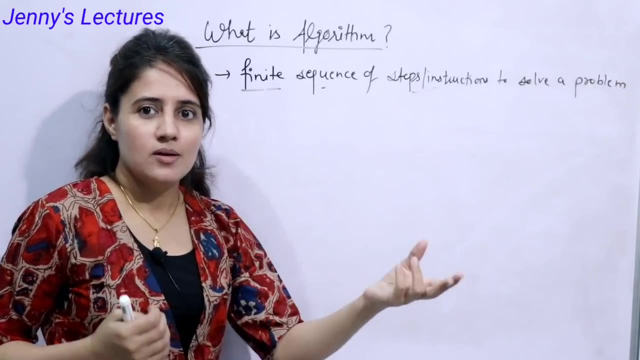 all. you can write algorithms. simply, If you want to update something, update in that algorithm and once finalized the design phase or the algorithm, then start implementation. Right, So you can say, to design better programs, algorithms are required. So I hope you got. 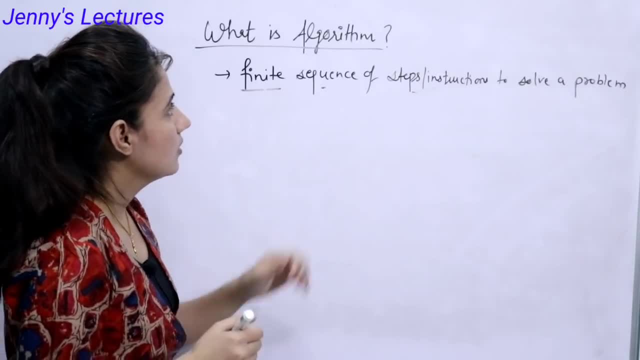 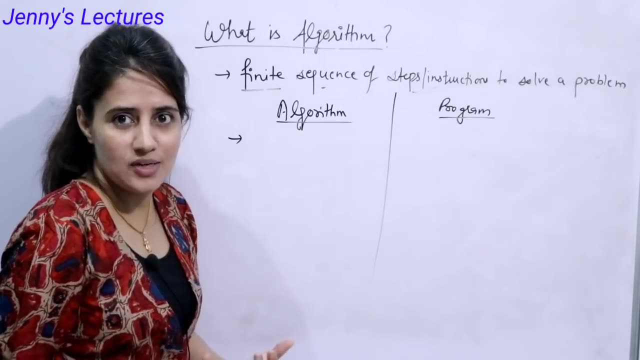 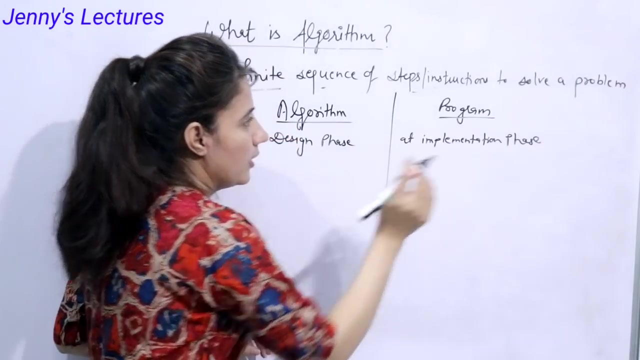 it why you need algorithms Now, if we discuss the difference between algorithm and program. So first, already we have discussed these are required at design phase and this is what actual implementation. So these are required at implementation phase. Now I hope everybody 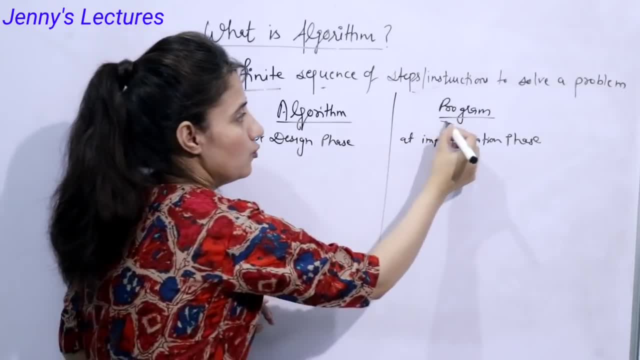 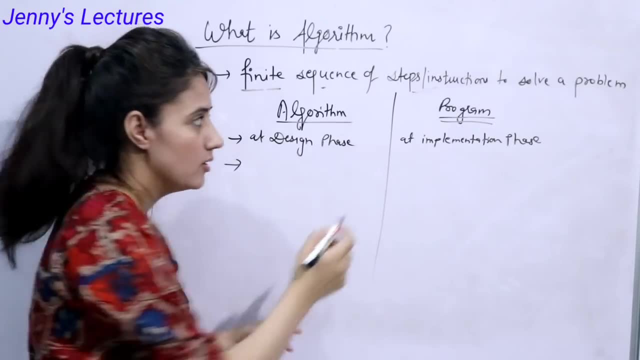 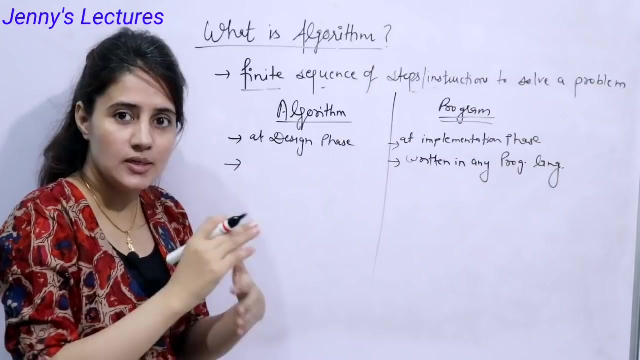 have seen programs, right? So In which language? So these programs are written in any programming language, like C, C++, Java, Python or any language, right? So these are written in any programming language, right? And they are required to follow that proper syntax of that language, right? Like if you are writing. 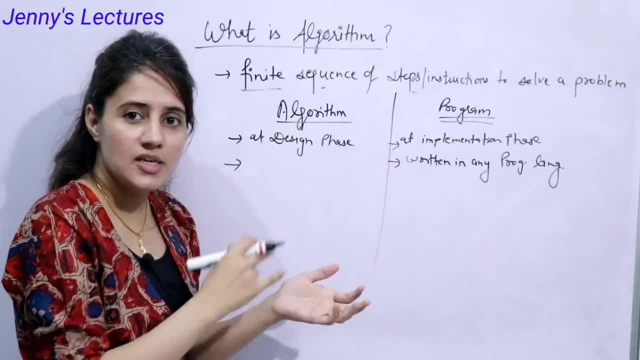 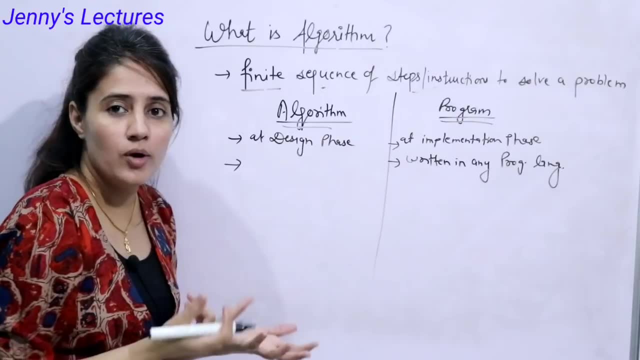 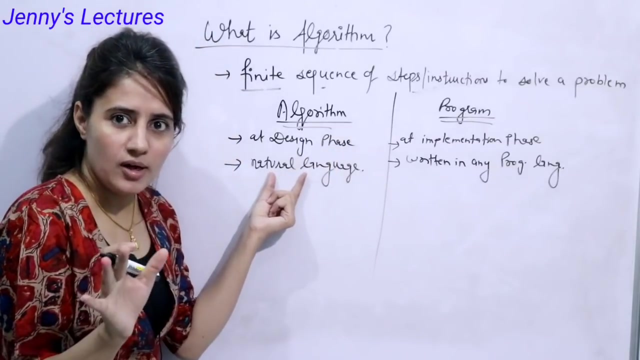 in C language then how to take input using printf and scanf, in C++ using cout and cin, like this right. But here to write algorithm you require what Natural language, Like simple English language, you can use, right, So algorithm can be written in any natural 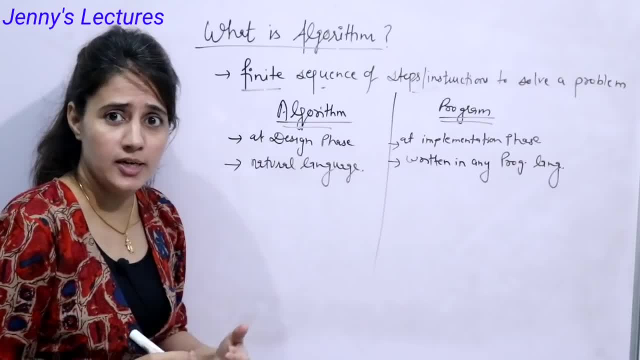 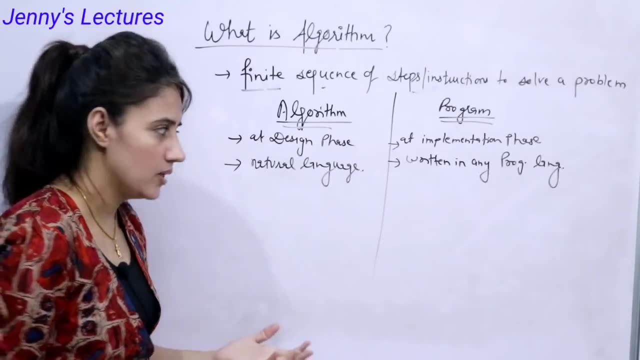 language. It is not like that, like this. you have to follow some proper syntax and rules and all. But yeah, to some extent a proper format is there to write algorithm right, But there are no strict rules or some syntax and all. 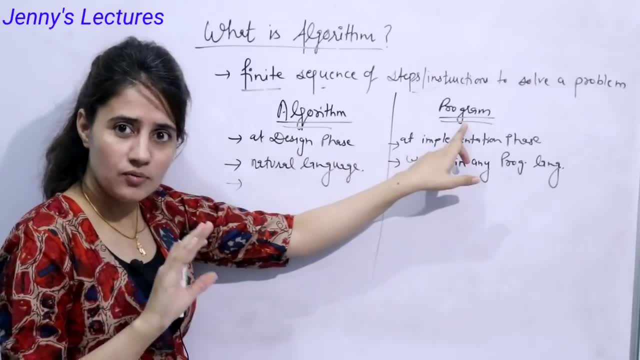 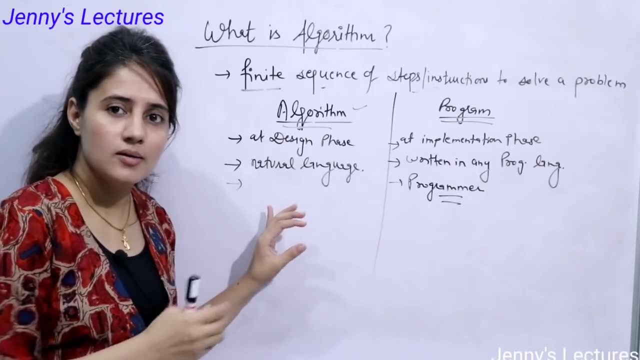 Next thing is like programmers will write programs, Now who will write algorithm? That same example: that construction of a building. right, So it is written in C, C++, C++, C++. that construction of a building. To design map, you go to an architect, That architect. 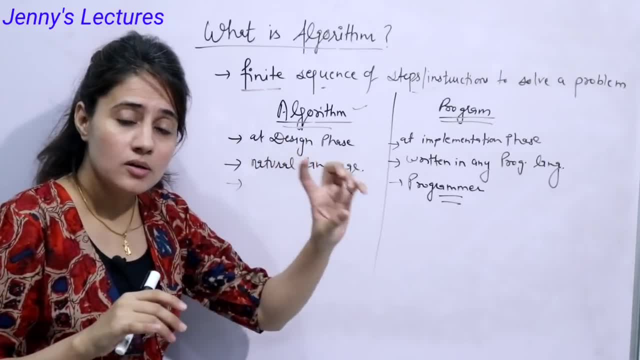 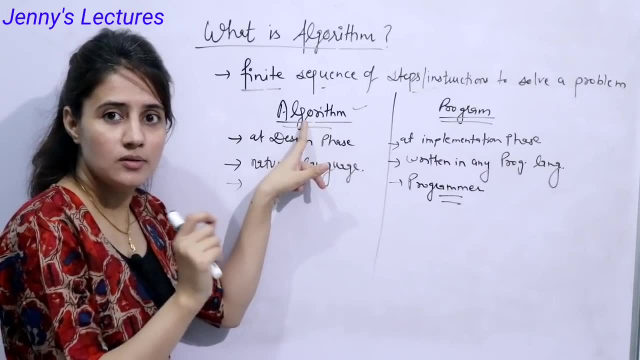 will give you map of that building. Why? So because that person is having knowledge of that field right. So who will write algorithm? The person who is having the domain knowledge for which you want to implement a software, right The person should have knowledge of. 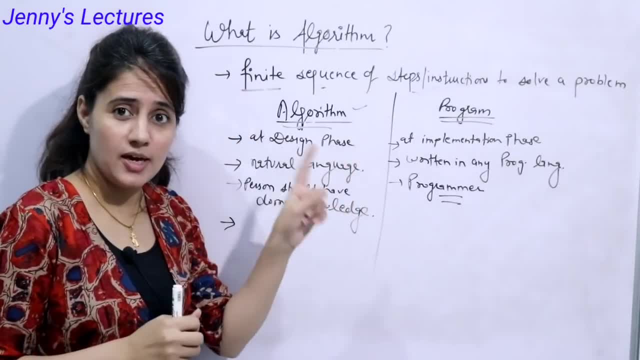 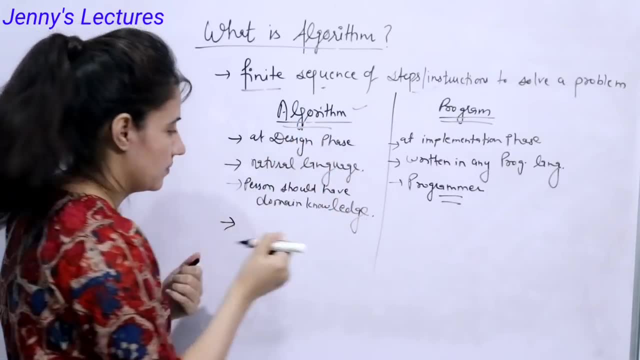 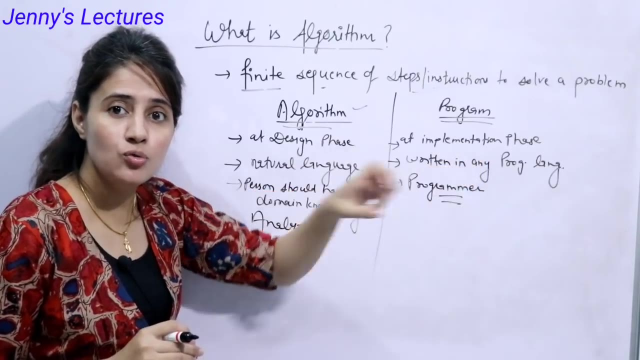 that domain. Now, next is see as the subject name design and analysis of algorithm. Analysis of algorithm, right? So we analyze algorithms, right? And what about programs? Program are at implementation phase. Then we are going to test these programs. Obviously we are.